Many, many, many of you probably have heard the term standard deviation A lot of times. you know if you're in a class or in college or something, or even in high school. maybe your professor might tell you, okay, the grades in the class where the mean was 75, or the mean 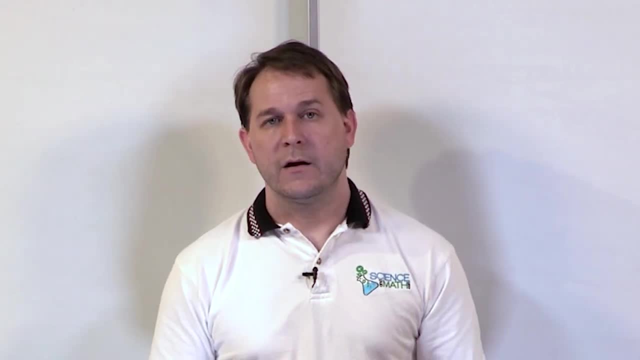 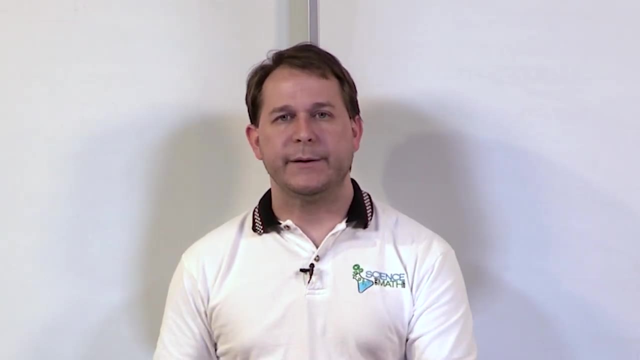 was 80, and the standard deviation was 10 points. right, And many of you have heard that but don't even really know what standard deviation of 10 points means. We're going to clear that up here. Much like the mean and the variance were extremely important central topics that you'll 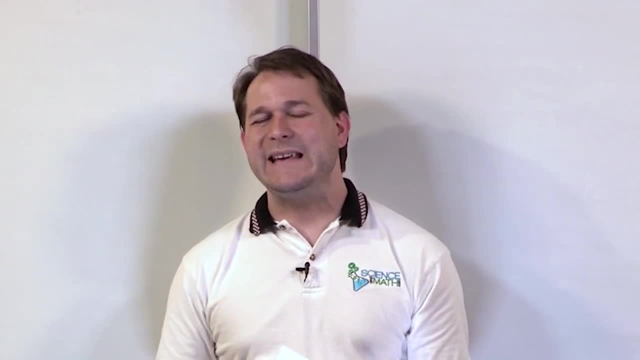 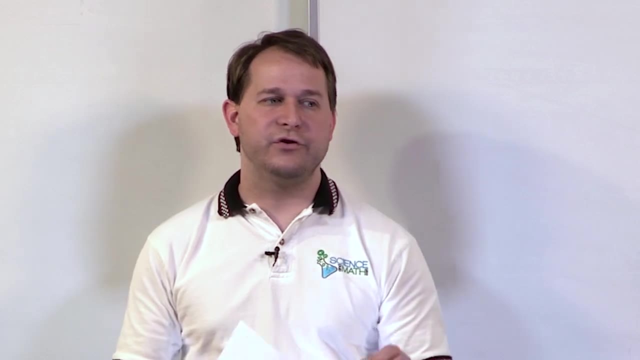 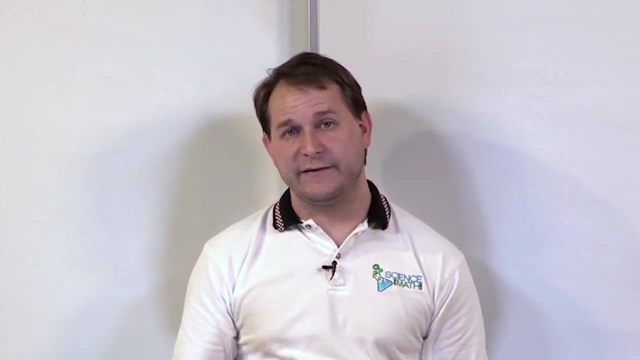 just see over and over again, the standard deviation is even more common than the variance when using and really describing sets of data. And again, the purpose of it is to measure the spread of the data. So let's walk down this logic and I'll explain how easy standard deviation is. 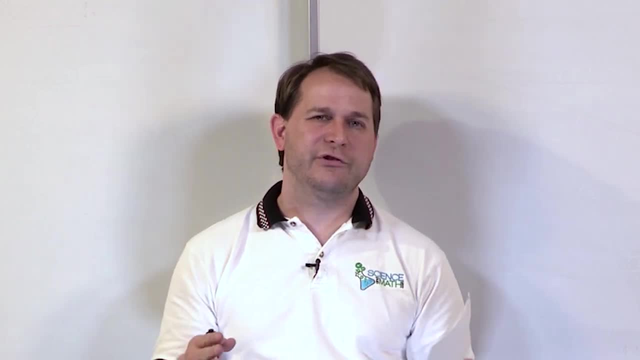 to understand. But as we talk about it, just think to yourself: okay, we're just trying to describe the spread of the data, So that's what we're doing. Now, recall that we're talking about the spread of the data, So we're talking about the spread of the. 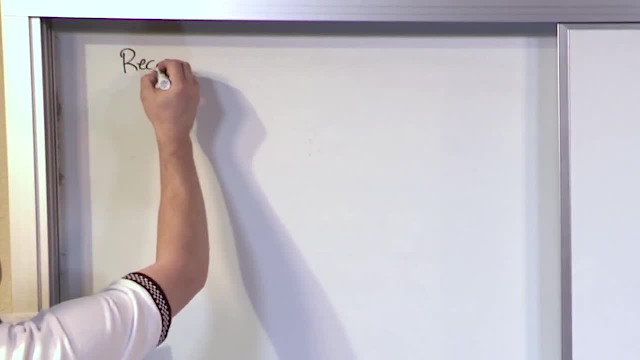 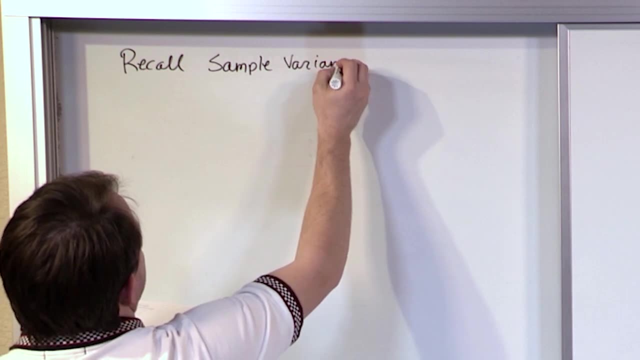 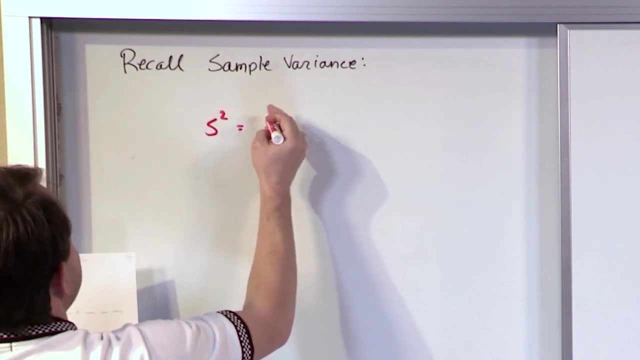 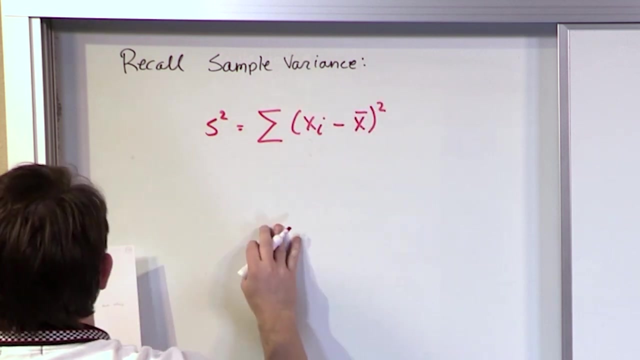 data. So recall, I will say recall, we've already learned the sample variance. The sample variance- and that I will change colors for, And that was denoted- s squared is the sum of the data points minus the average value squared over n minus one. We've done that before. 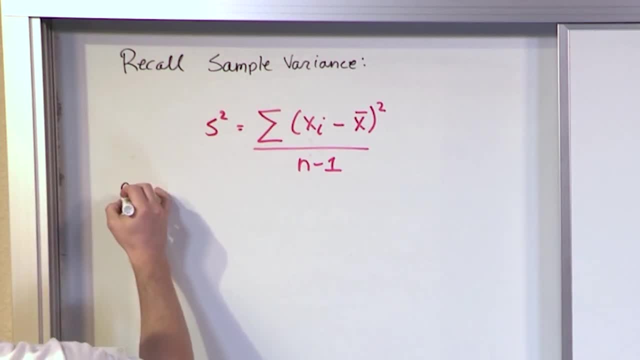 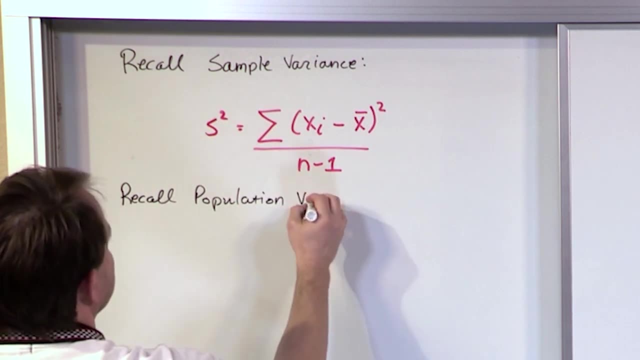 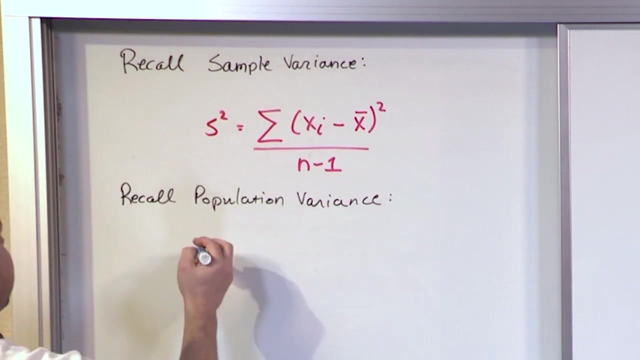 We understand that Great. Now recall also the population. There's a reason I'm writing all this down again, So just kind of bear with me. The population variance, I'll go ahead and just rewrite that again. We called it sigma squared And it was the sum of all of the data points. 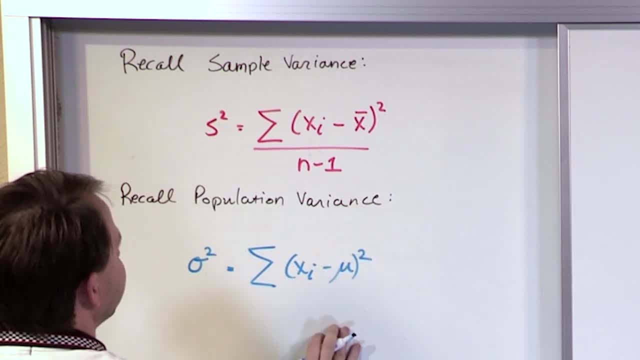 minus the population mean that's what that is: everything squared just like before, And instead of n minus one. we'll just write it down again And that's what that means. So that's what that one it was in the total number of people or items in the population. This is what we've. 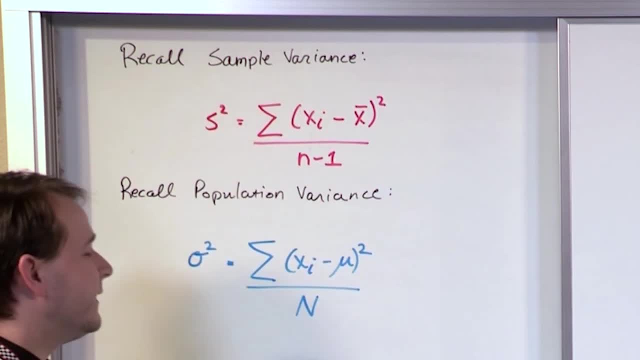 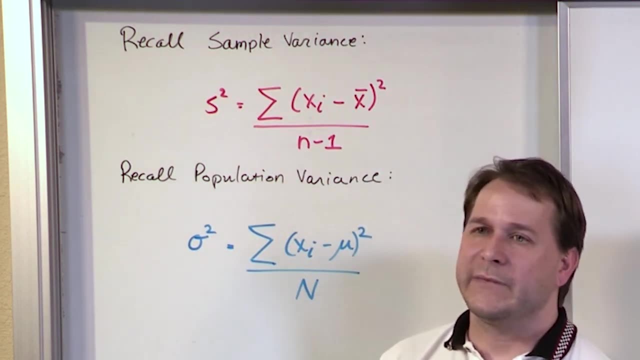 learned before. These do measure the spread of the data. They do, But the problem, if you want to call it a problem, is that because we squared everything, it does measure in a relative sense how spread the data is. You can look at two variances of two different data sets and figure. 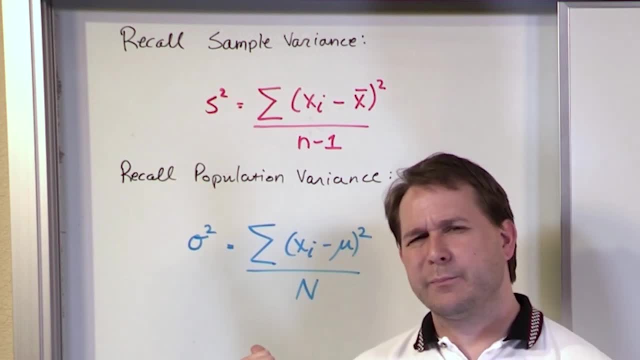 out which one's more spread by looking at which one's larger. But the problem is, we've squared all of our data points. So because we've squared it, all the differences, we've squared everything. So when we get a variance of 10.9, or if we get a variance of 5, what does that mean? Because 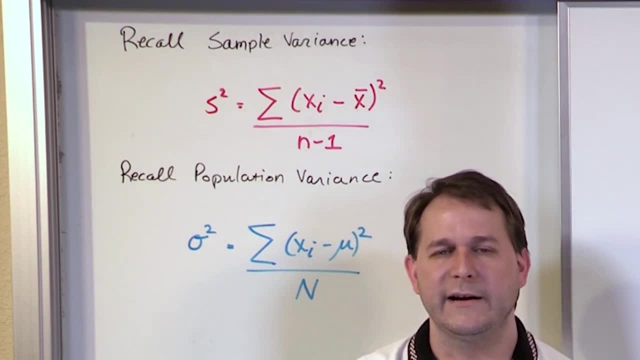 everything's been squared. it's not in the units of our original data points anymore. In other words, if I calculate the variance of the grades in a classroom, like I may have some students in a class and the average value or the mean of everybody's grade might be an 80, right And I 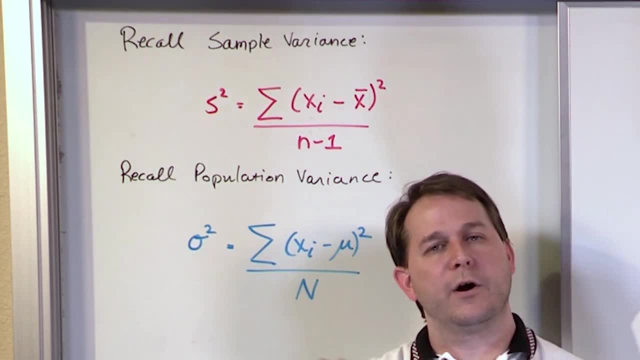 might calculate the variance of all that data. And I might calculate the variance of all that data to try to figure out how, spread apart, everybody is about the mean. And let's say I calculate the variance, that ends up being 15,. right, If I calculate the variance of 15,? is that 15 points? 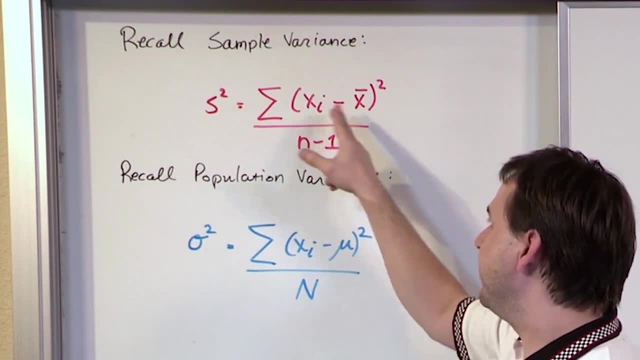 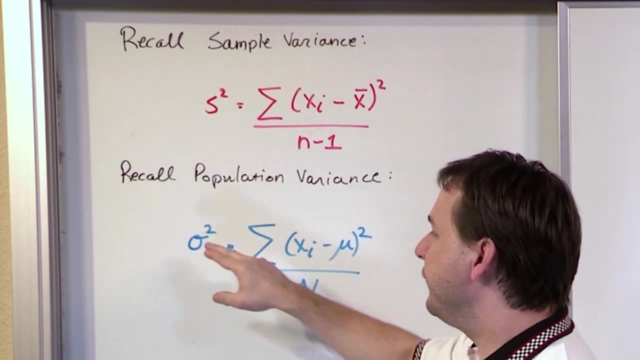 like 15 test points. No, it isn't because I subtracted everything from the mean, but then I squared it. So that's kind of why everything is labeled out here with a square. It's reminding you that the calculation you did does represent how spread the data is, but I've squared everything. 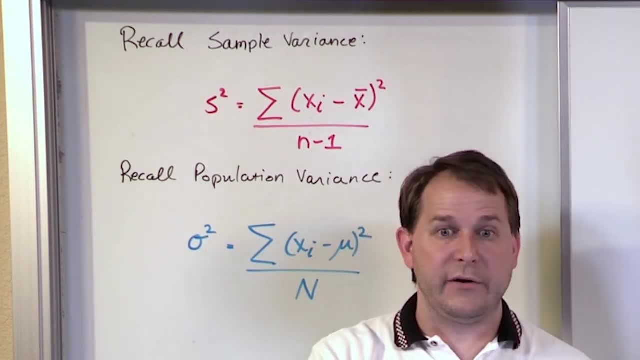 And so I can't really say that when I say the variance of 10, talking about the grades, that it's 10 points variance plus or minus the mean, because everything has been squared. So what we're going to do is fix that. 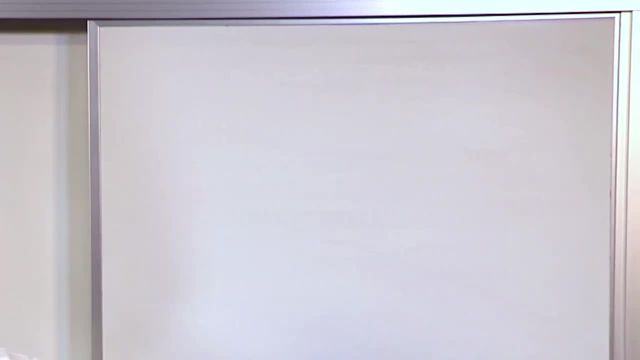 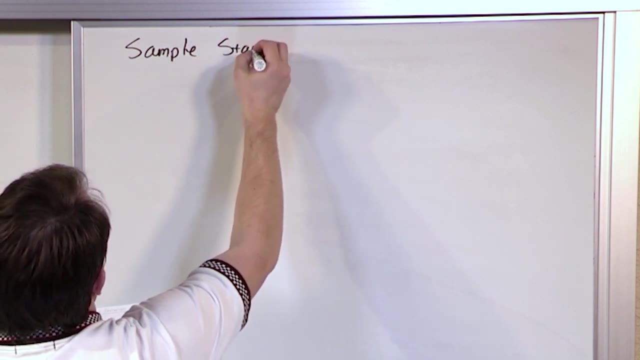 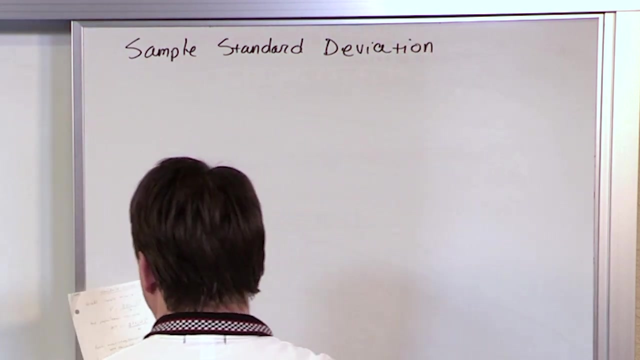 little problem right now And I'm going to go off to the other board and write that down. So what we do is we have the sample standard deviation And it's so simple. once you understand what it is, it's great. The sample standard deviation is labeled. let me go ahead and do this. one in red. 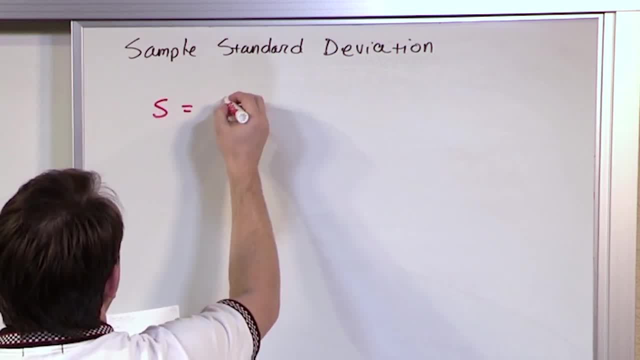 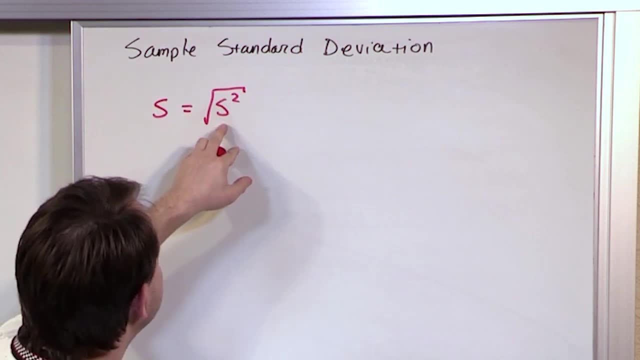 is labeled S And it's literally the variance that we know how to calculate already, but we just take the square root of it, See, because the variance is kind of like a calculation that involves all the squaring of all of the differences of the data points. So if we just take the square root of that, 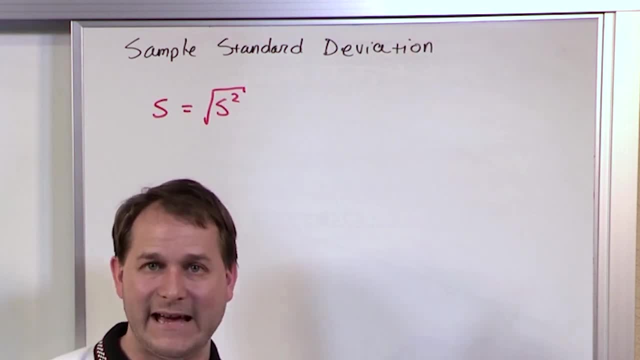 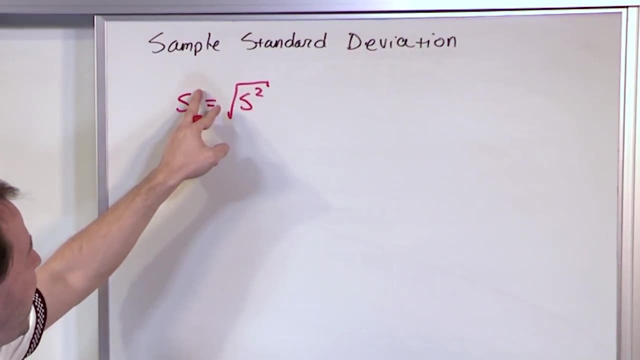 then we eliminate the squaring business. We do the square rooting at the end, obviously after we've calculated the variance here, And then from that we get just S. There's no S squared here anymore, When you see S by itself. 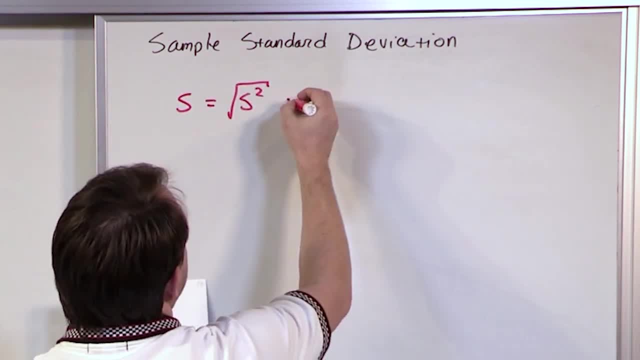 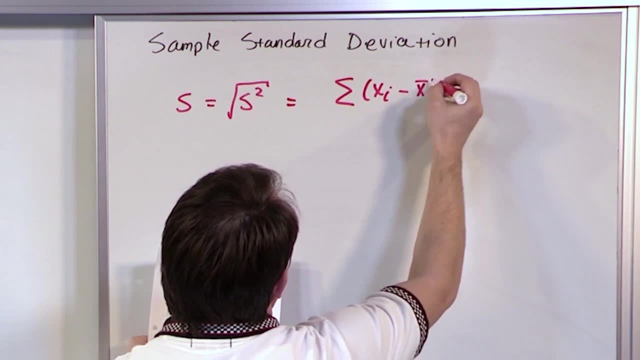 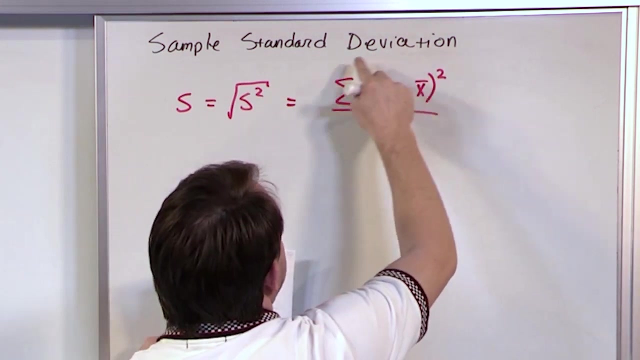 you refer to it as the standard deviation. So if I had to put it down in all of its glory, it would be the sum of the data points xi minus the average value, squaring each difference like that, divided by n minus 1.. This calculation, right as it sits, is the variance. It's exactly. 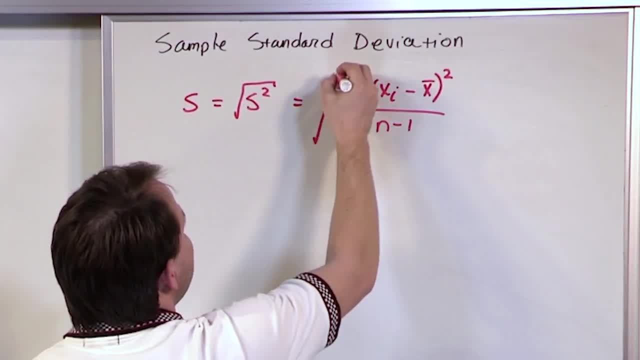 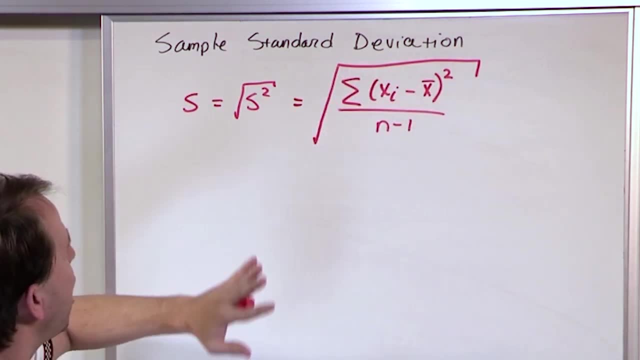 what I've written here. okay, So to calculate the standard deviation, you do all of the squaring business, all of that, and then at the very end you take the square root of the whole thing. So when you do the square rooting business, at the end you don't call it the variance anymore. 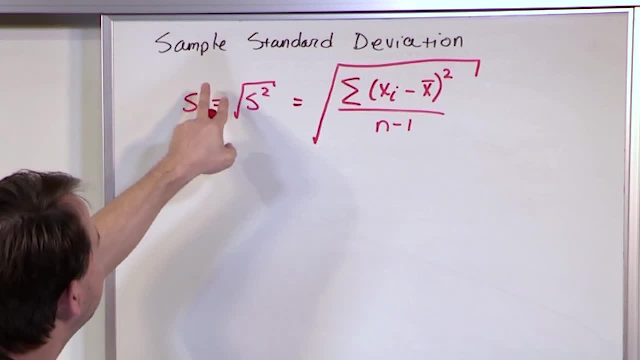 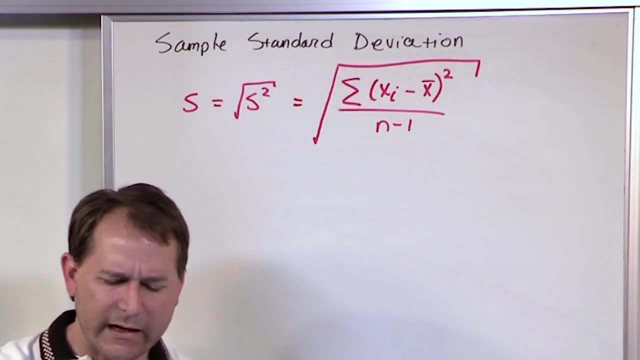 You call it the standard deviation. You use the same letter S, but you don't put a square over there, And this is a reminder that you don't have this squaring business anymore. So if I have, for instance, a classroom where the mean is an 80,, all right, and the standard deviation. 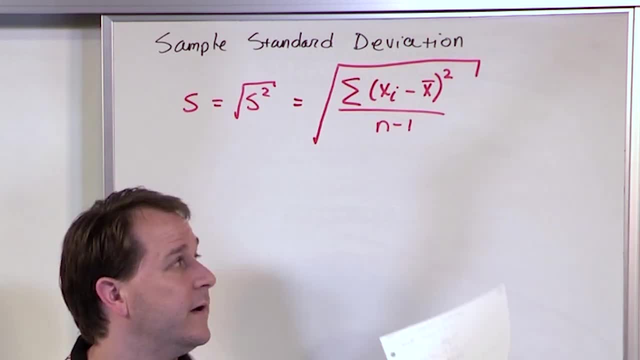 after I calculated, by doing all this business with the square root at the end, the sample standard deviation. if the standard deviation is 10, then the units of my standard deviation match the units of my data set. So if I'm talking about points in a classroom grade, then the mean is 80 points and the standard deviation of 10. 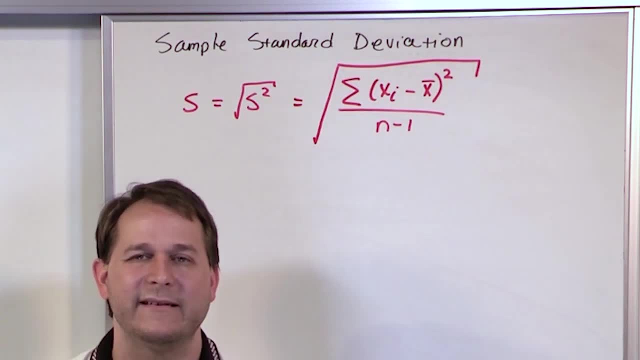 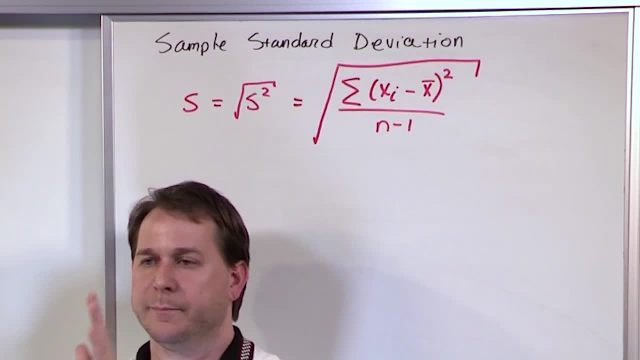 the data did. It means that one standard deviation on the plus or on the minus side of the mean it tells me that a good chunk of the data, a nice large amount of the data, falls within that amount of the mean. So if I have a standard deviation of 10 points on a test, 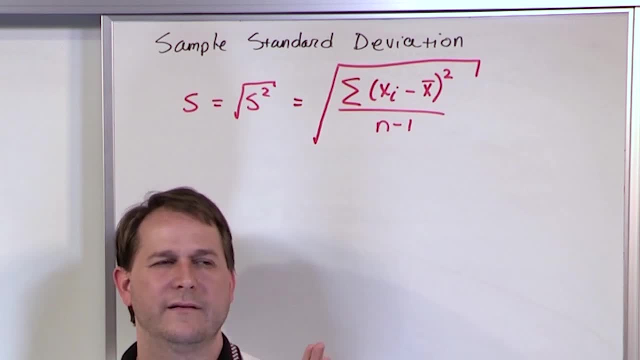 and the mean was an 80, that means lots of the points, lots of the grades in the room fell between 70 and 90, because that's 10 points plus or minus. It's the standard deviation where 10.. If the standard deviation were 15, then it would be 15 points around the mean Most. 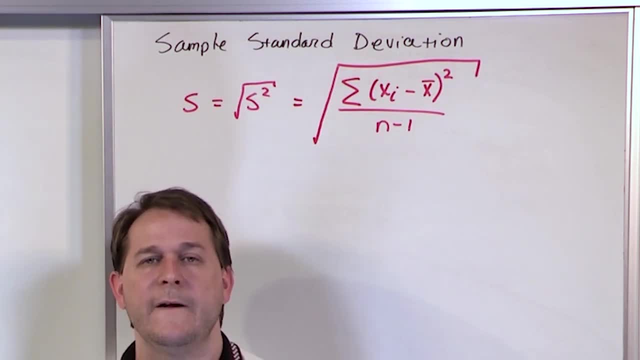 of my data fell around 15 points around the mean. So the standard deviation to me actually makes a whole lot more sense to really talk about than the variance. You have to introduce the variance first, because that's where the genesis of the calculation comes from, And there are lots of. 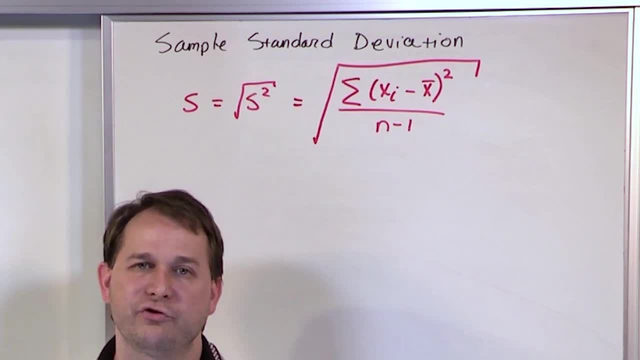 equations and statistics that use the variance. But whenever I'm describing a set of data to some person and I'm trying to give them a sense of how spread out it is, I'm almost always going to use the standard deviation, Because I can tell them hey. 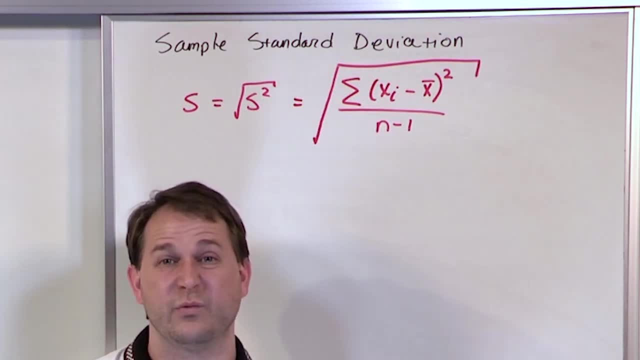 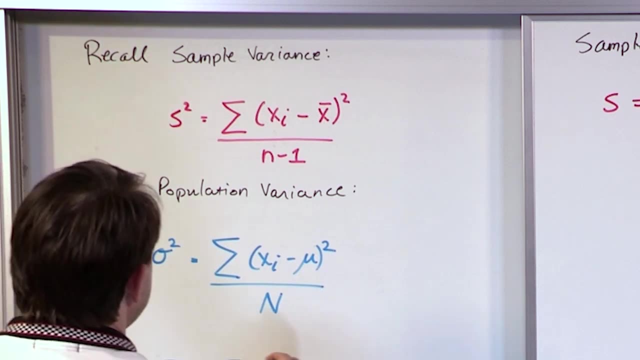 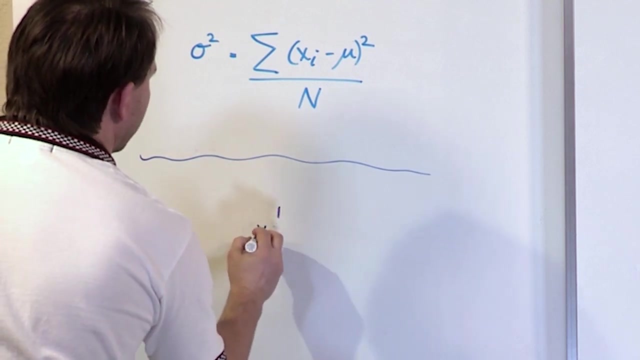 the mean of the exam was 60, but the standard deviation was 30 points. What does that mean? That means that if I were to do that- let me just kind of go down here- If I had a really kind of poor result on my test and I said the mean right x bar was 60 points, 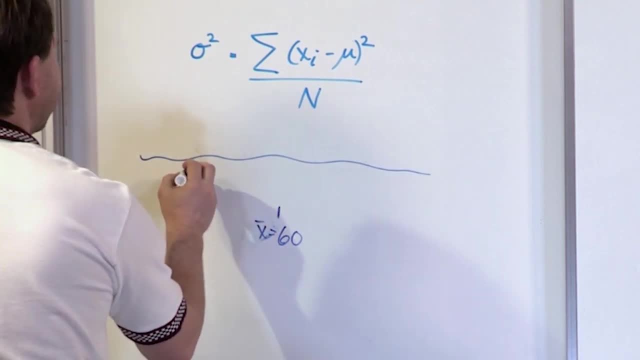 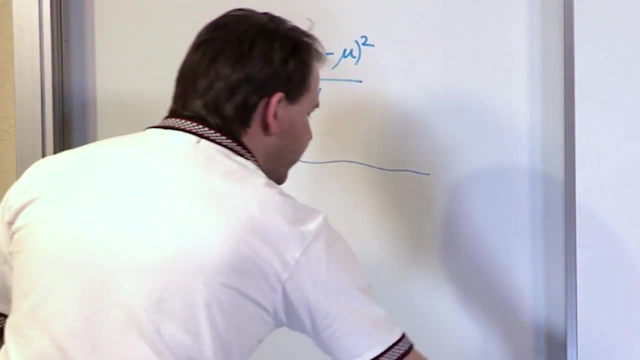 right. And if I said the standard deviation- in this case let's say the standard deviation s- was 30 points, then what does that mean? That means that here's 60. So 70,, 80,, 90. So here's. 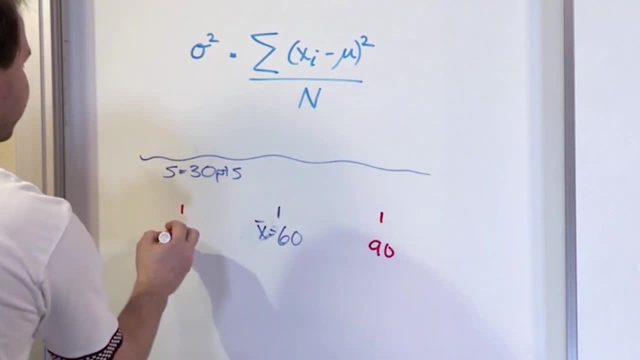 90 here. You subtract 30 up here, that would be 30 down here. That means that a large amount of my data fit into this window. When I have a standard deviation of 30 points, what it means is 30 points. 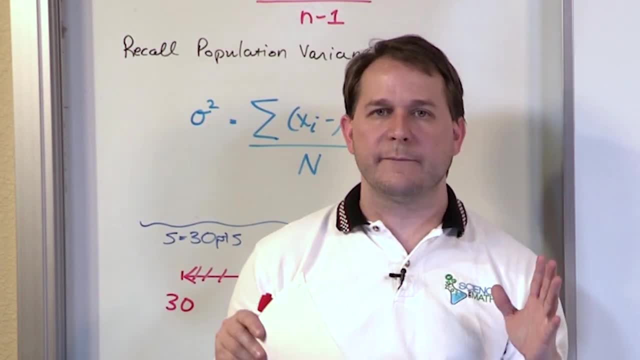 around the mean. That's what it is. It means that a good chunk of my data as a eyeball, as a calculator, is going to be a good chunk of my data, And that's what it means. So if I have a 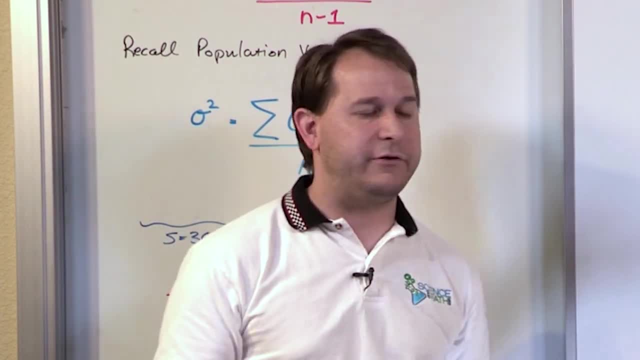 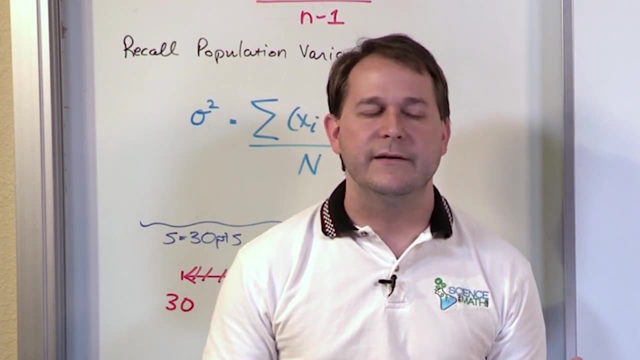 standard deviation of 30 points. what does that mean? That means that a large amount of my data actually falls between plus or minus the standard deviation in reference to my mean. So it makes a lot more sense to talk about standard deviation than variance in a lot of cases, because I can. 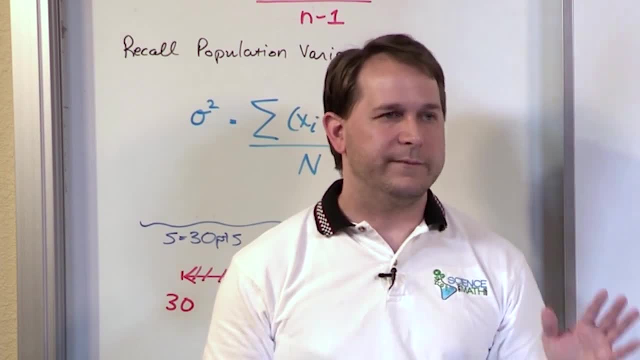 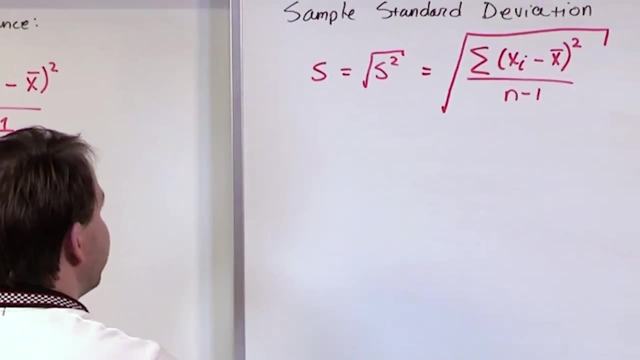 tell you the standard deviation was 10 points or 20 points. The units of my standard deviation are the same as the units of my data set. all right, So let me go and write the rest of this down and we'll talk about it even a little bit more. Let's say that the this is the sample standard. 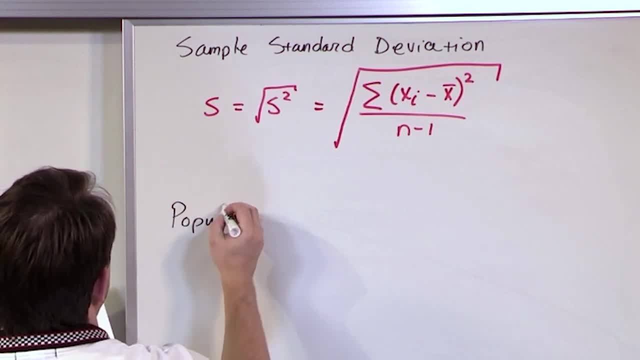 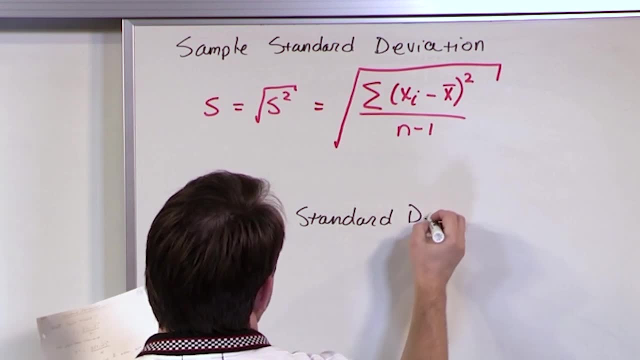 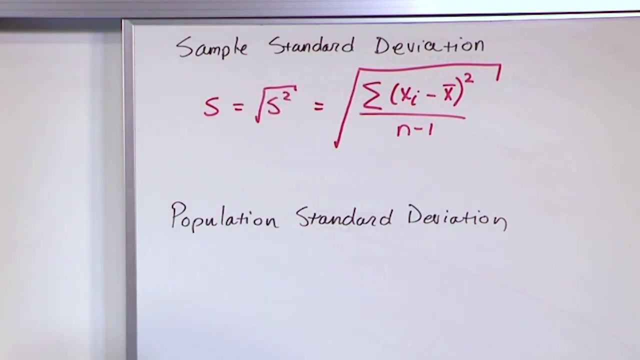 deviation. So let's say we have- let's say we have- a standard deviation of 30 points. So let's say we have the population standard deviation right. So if this is the sample standard deviation, what do you think the population standard deviation would be? Well, first of all, 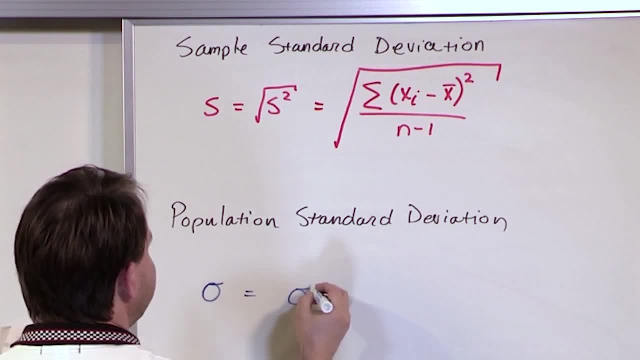 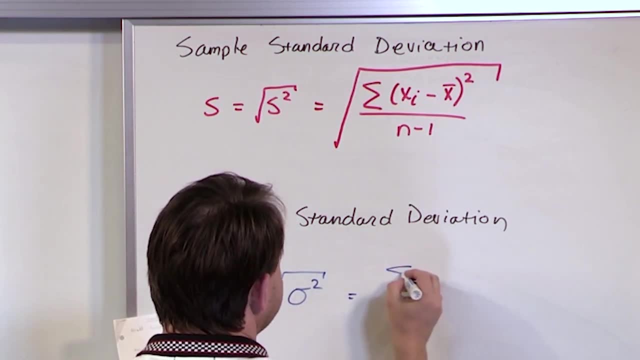 you're going to use the symbol sigma to represent it And you just take the population variance that we know how to calculate and you take its square root. So really it's the same sort of thing. It's the sum of the data values minus the population mean, each one of. 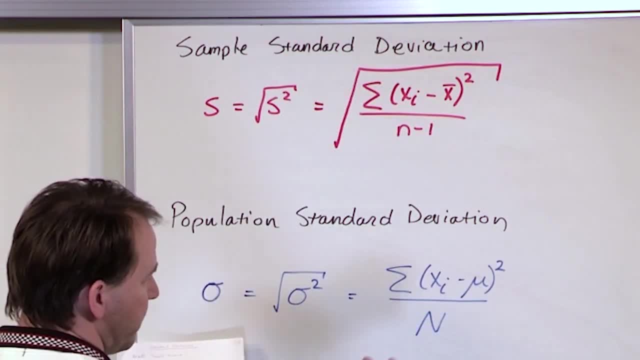 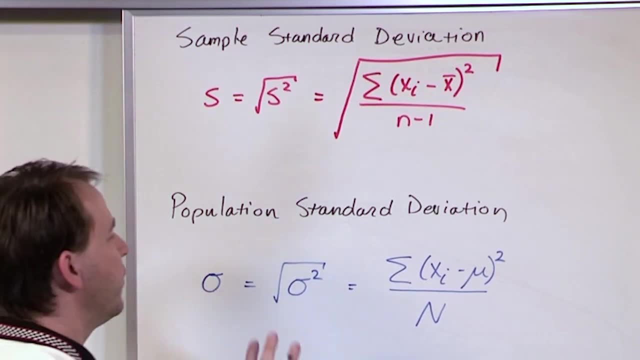 those differences squared, divided by the total population number of items you have. This, as it stands, is calculating the population variance, exactly what we've talked about before. But to make it a standard deviation, we wrap the whole thing in a square root. do that at the very very. 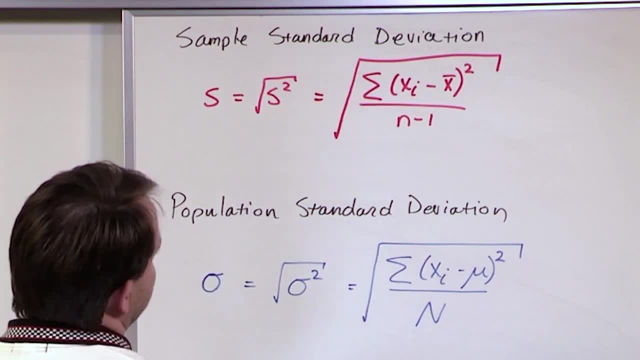 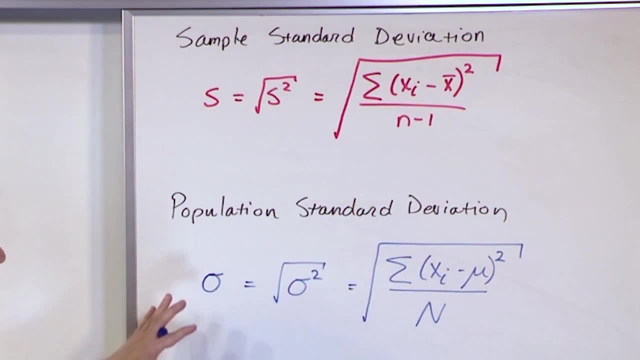 end. So these two items, the sample standard deviation, which is just the square root of the sample variance, and the population variance, are the same sort of thing. So let's say that the population standard deviation, which is the square root of the population variance, are extremely. 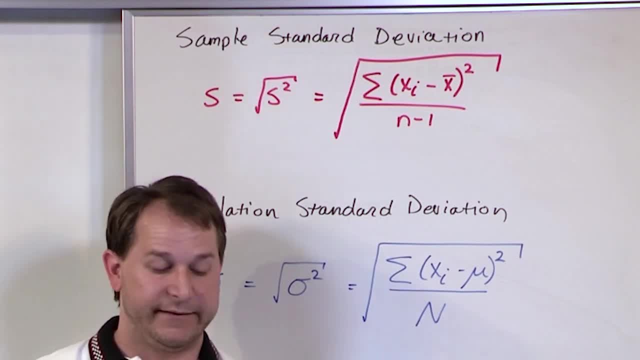 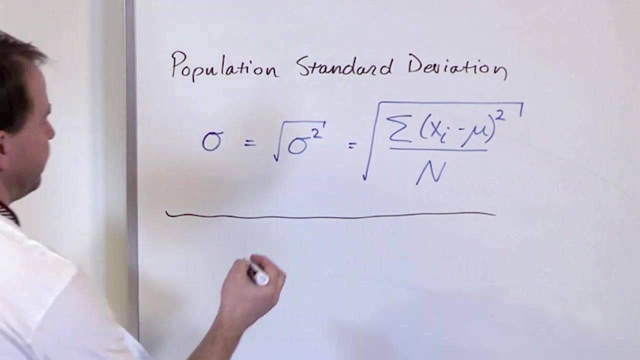 central, important topics in statistics. I cannot stress it enough. I'm going to do some examples to show you how to calculate this with a real data set, But just to kind of just drill it home one last time. let's say I had some ages of people in a classroom right And I told you that the 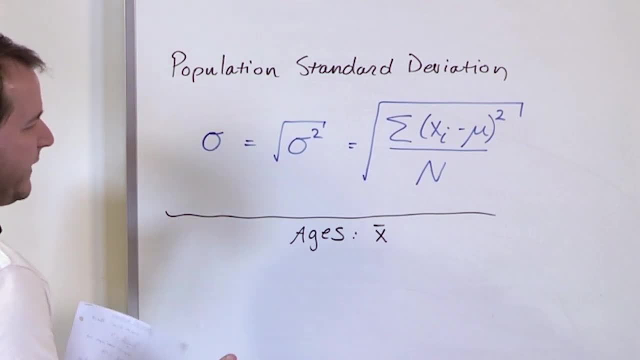 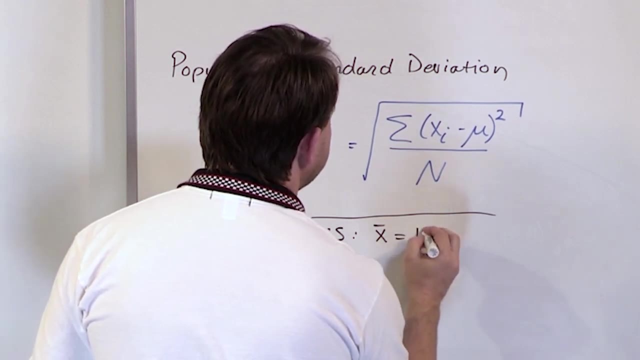 mean of the ages in the room. let's say I have like 20 people in the room. the mean was, let's say, 15 years old. right, That tells you where the middle of the road, like roughly where the middle. 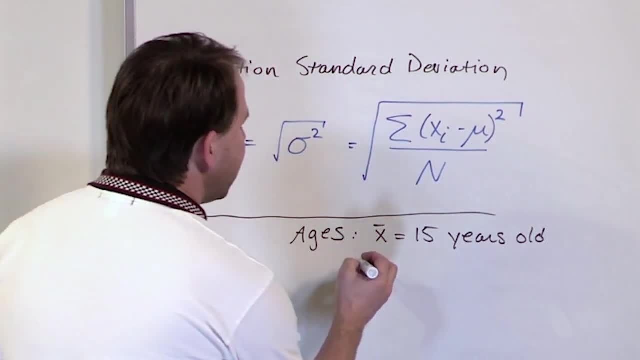 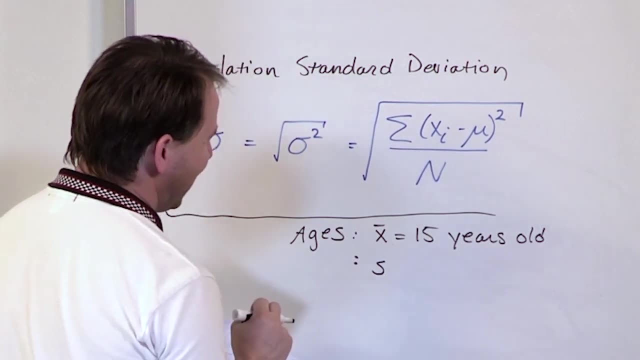 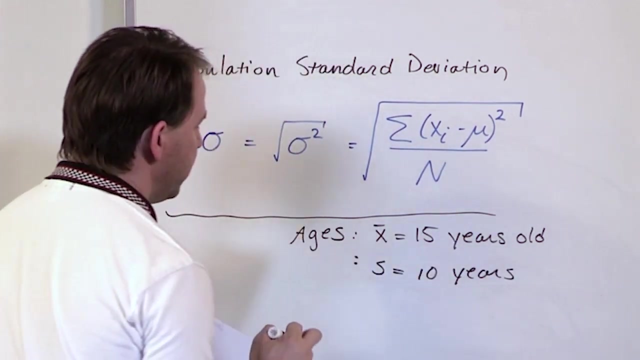 of the ages lie of everybody in that room, all right. And then I tell you- because this is a small sample of people, let's say in the room- I tell you that the standard deviation S is around, let's say 10 years or 10 years- Then what you should visualize in your head is that if 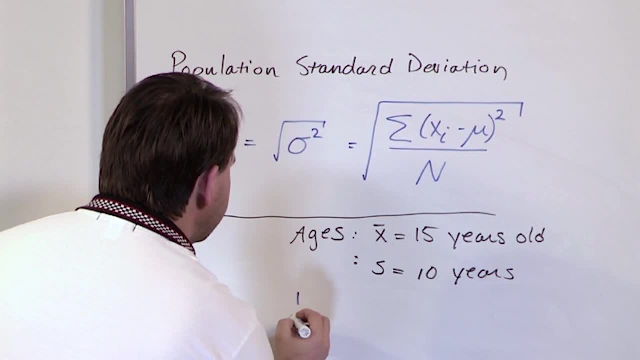 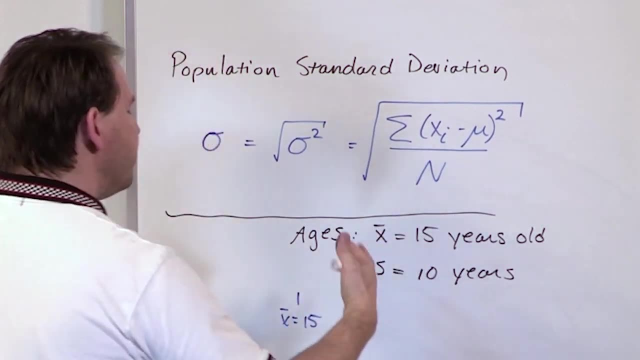 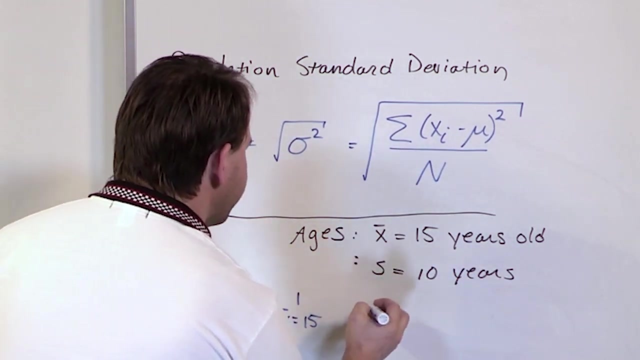 everybody here. is everybody in the room, then the mean is going to be 15,, right, But the standard deviation tells me that, on average, most or a good chunk of my data falls plus or minus 10 years around this mean. So that means 10 years plus over here would be 25, and 10 years minus over here. 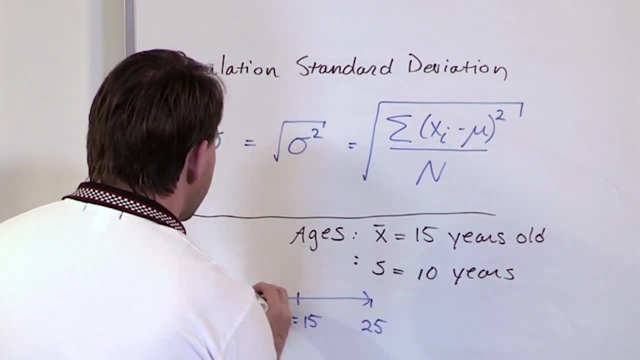 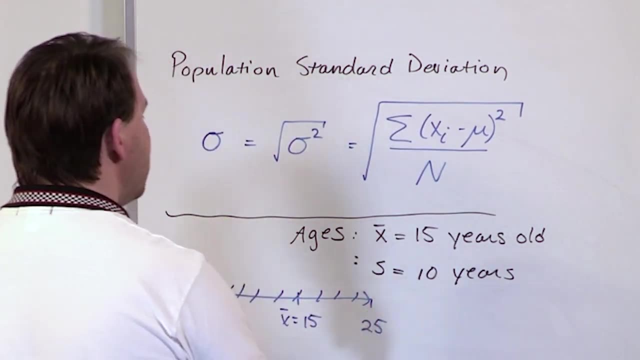 would be 5.. So then, in between these values here a good chunk of my data lies. Now. some of the data does lie out here and some of the data does lie out here, but a good chunk of it lies within plus. 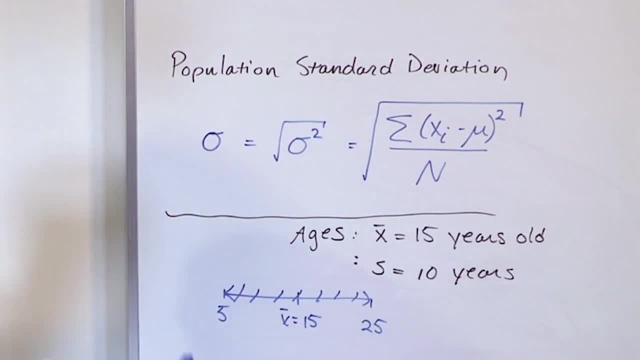 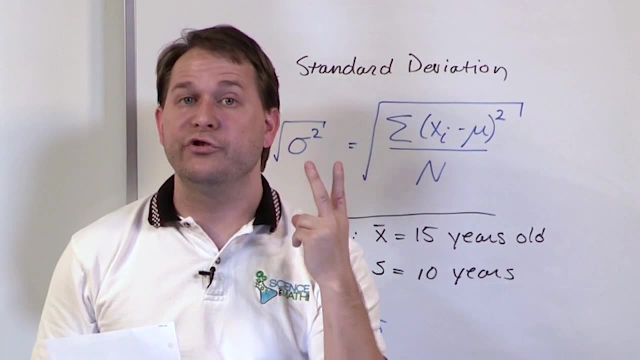 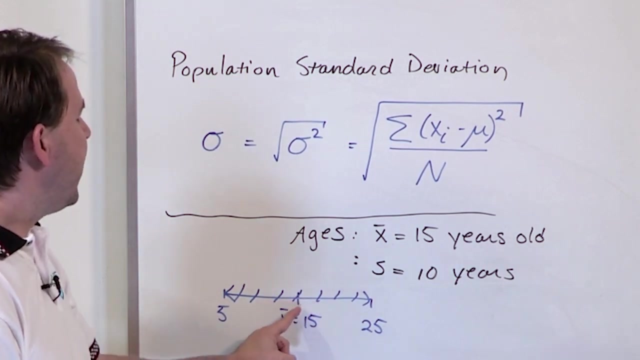 or minus 10 years of the mean. okay, In contrast, I'm not going to draw another picture. if the standard deviation were, let's say, 2 years, right, If the standard deviation were 2 years, that would mean that the mean would be here and I would be plus 2 years and minus 2 years, so up to 17, and 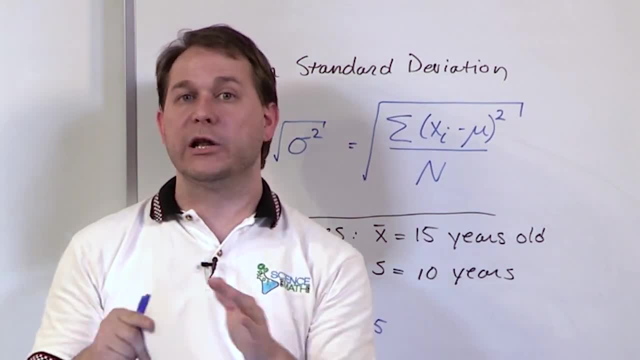 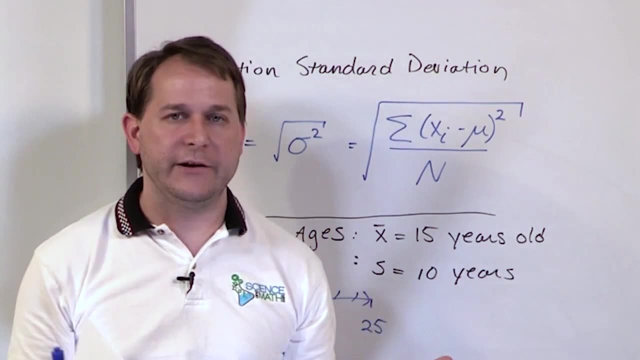 13, very tightly packed data. It would tell me that a lot of my data falls within plus or minus 2 years of the mean, which is 15.. So I can easily give you two pieces of information about a data set- the mean and the standard deviation- and you can instantly get an idea of what that data set. 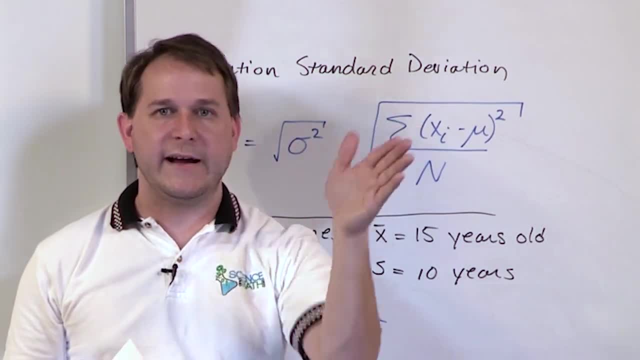 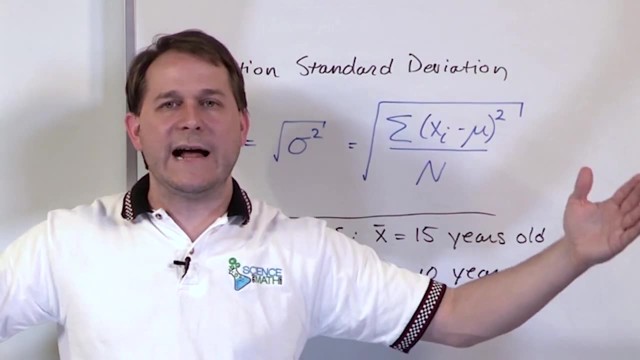 looks like The mean helps you visualize where the center of the data is. The standard deviation tells you how broad it is right. If I have a very large standard deviation, then lots of values lie on both sides of the data set. So I can easily give you two pieces of information about a data set. 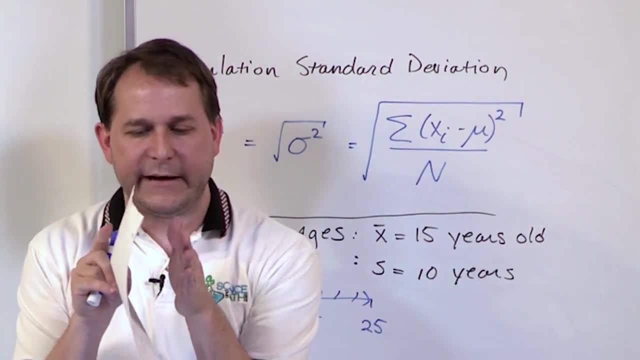 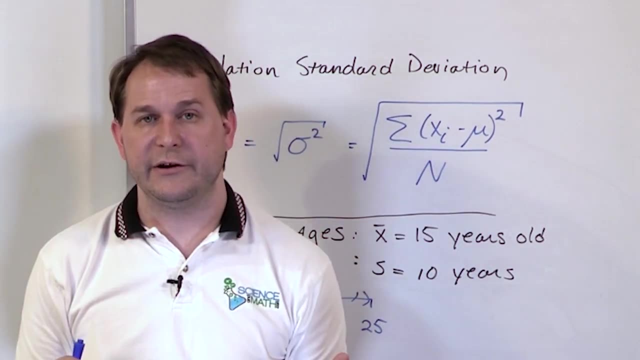 the mean and the standard deviation. If I have a very small standard deviation, then I have a very tightly compact data set, plus or minus, however many units your standard deviation is. So I've tried to give you some examples. I want you to internalize what this means, because it's so. 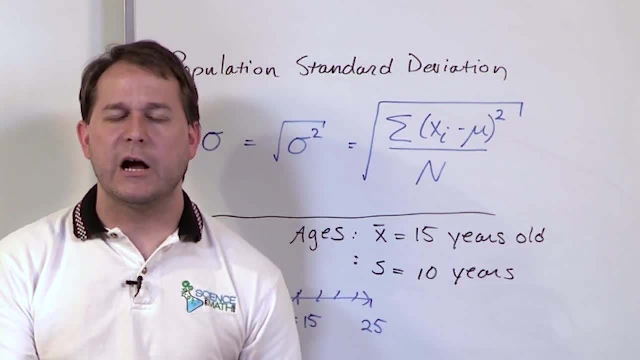 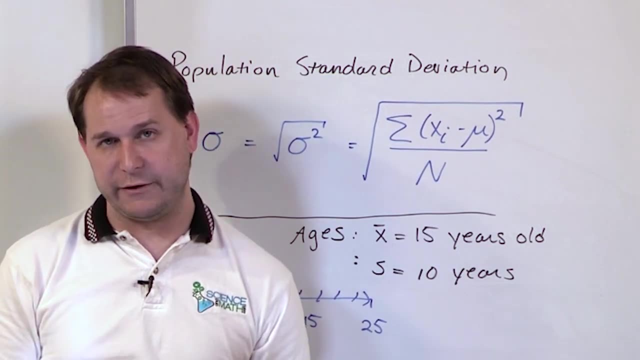 important for future lessons. Make sure you understand the concept behind standard deviation and then meet me on in the next lesson where we will go on and just do some calculations and show you how to calculate the standard deviation. The calculation is going to be a little bit more. 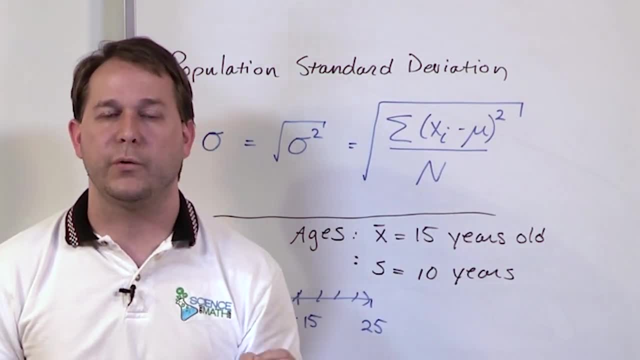 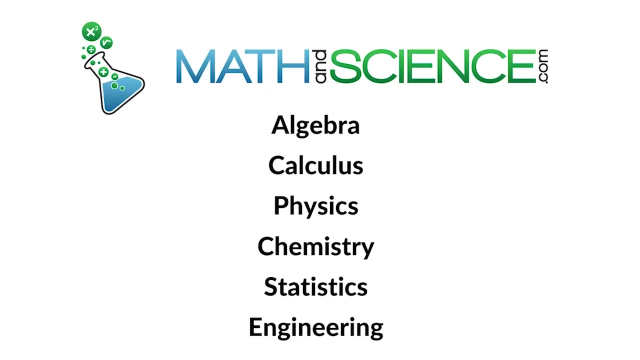 complicated and it's really the same as we've done in the last section, but I still think it's important for you to get some practice with it. So follow me on and we'll get some practice with calculating the standard deviation in statistics. Learn anything at mathandsciencecom.